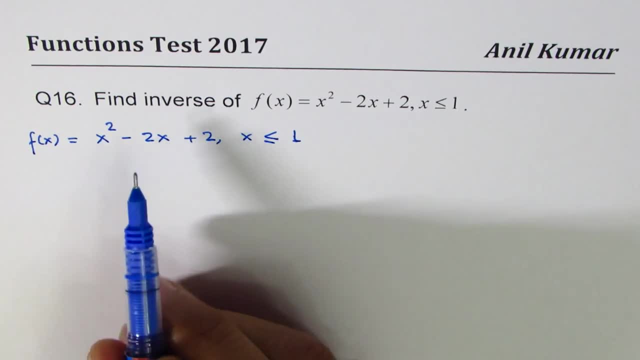 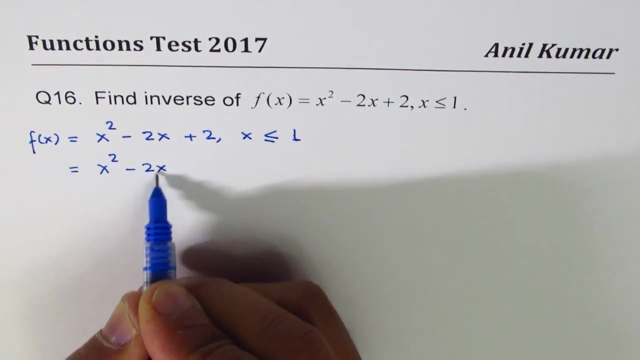 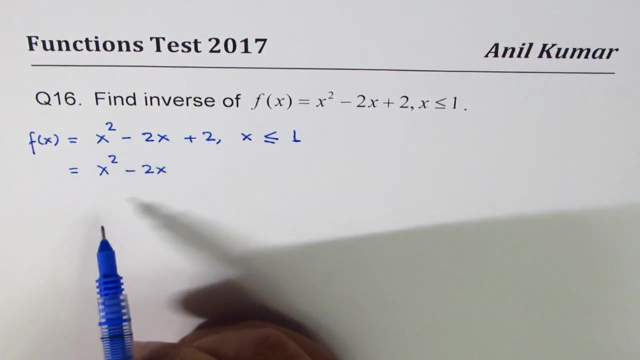 Now this is a quadratic equation, standard form. To find inverse, it is necessary to do what? Complete the square and write it in vertex form. So let's change the form first, right? So we have x squared minus 2x. If you don't change it to vertex form, you actually cannot find inverse, since there are two different x terms, right? 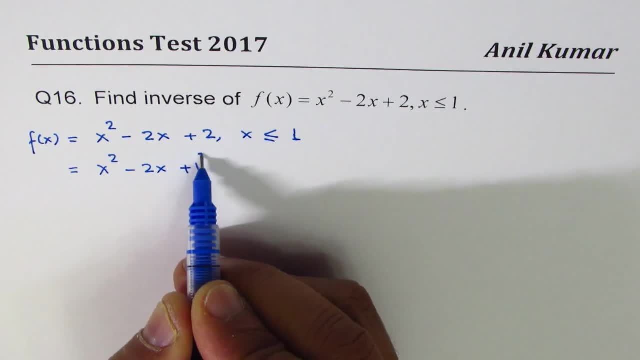 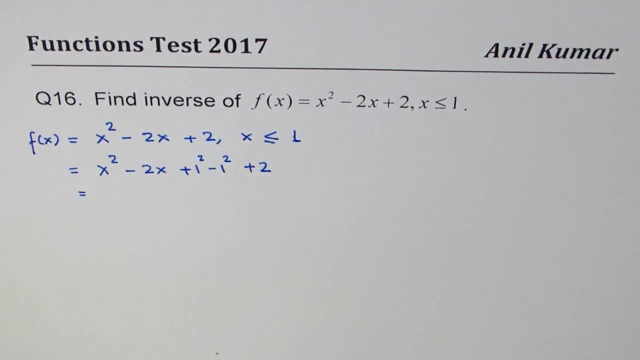 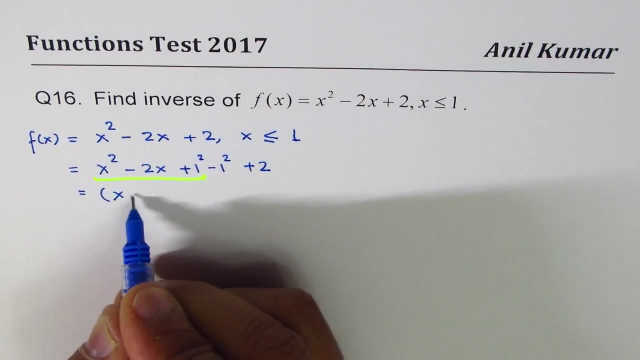 So half of 2 is 1.. So we will add and subtract 1 squared, Is it okay? And we have plus 2.. So we have plus 2 here. The first three terms will form a perfect square. right, These three terms form a perfect square. So we can write them as x minus 1 whole square. and then we have minus 1 plus 2, right, These two terms. and that gives us x minus 1 whole square, plus 1.. 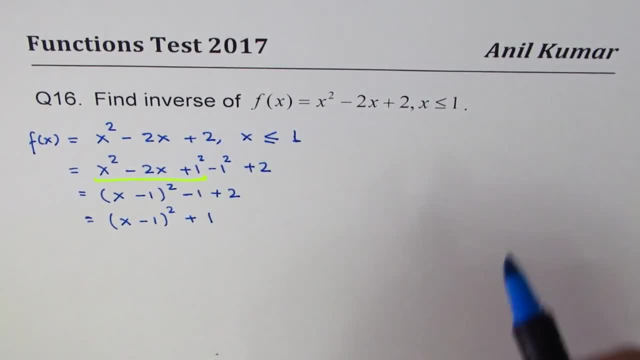 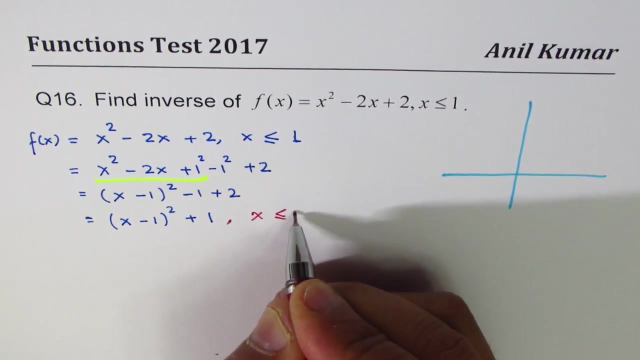 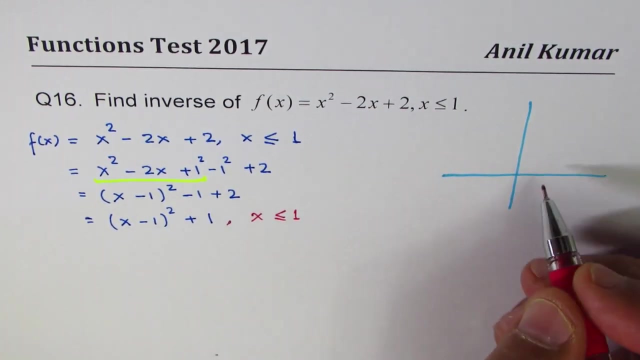 So let me sketch this function for you. So what we have here is we have a parabola and remember, the domain is x less than equal to 1.. Very important to understand. It has vertex at 1, 1, right? So the vertex is at 1, 1.. Let's say that's the vertex for us. 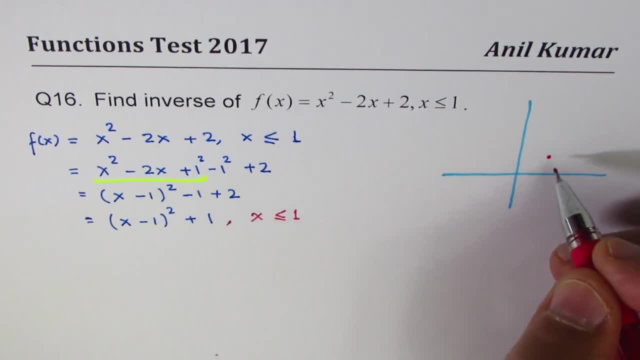 It opens up with steps of 1,, 3,, 5,, 7,, right, So it is 1 here. So next time it will be at 2.. This will be the point, So the graph of this function could be sketched as. let me sketch a dotted graph first. 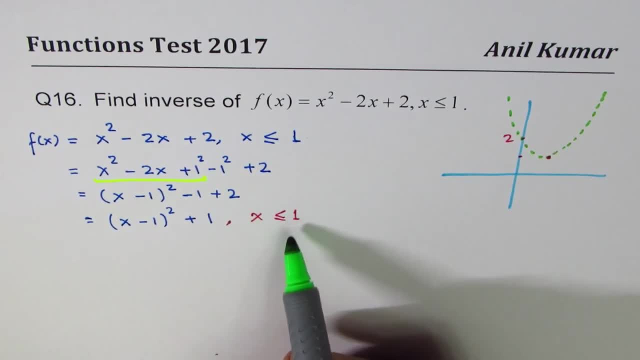 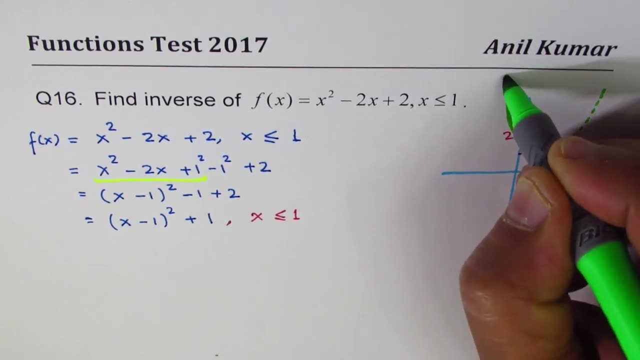 Okay, Since x is less than equal to 1, we are only considering the left side of this graph. That's important to understand, Do you understand? So that is what we mean. This is the part which is of our interest. 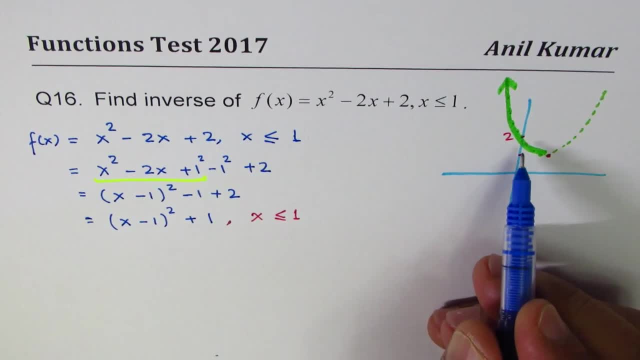 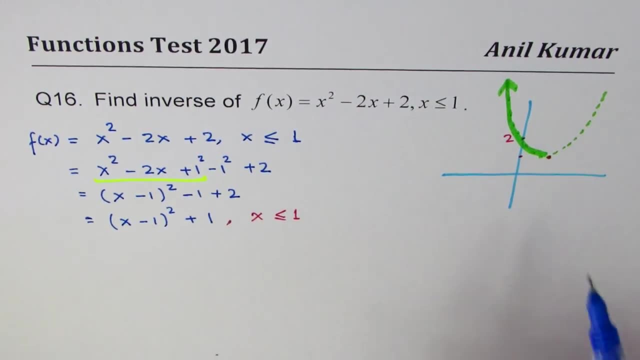 Is it okay? Correct. So x less than equal to 1.. We are trying to find its inverse. So when you try to find inverse, you have to reflect the graph on: y equals to x. What do you expect? You expect a square root function, correct? 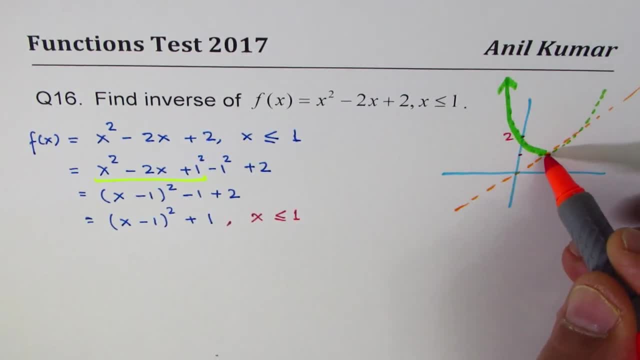 Which of this? so only one arm. Do you see that You expect this to be a square root function, which is kind of opening like this, Of course, correct. So this point is 0, 2.. It just becomes at 2.. Is it okay? 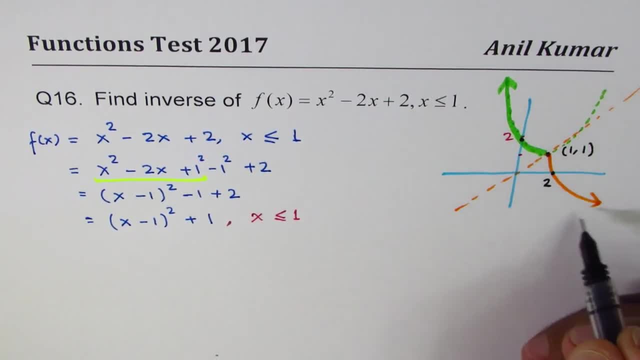 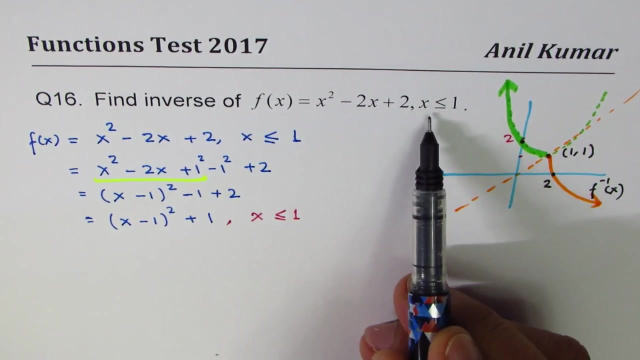 This is invariant, point 1, 1.. So that is the inverse of your function. This is inverse of the function. Now I have sketched all this To make you understand how to write inverse of a function when conditions are given, especially for the domain, correct? 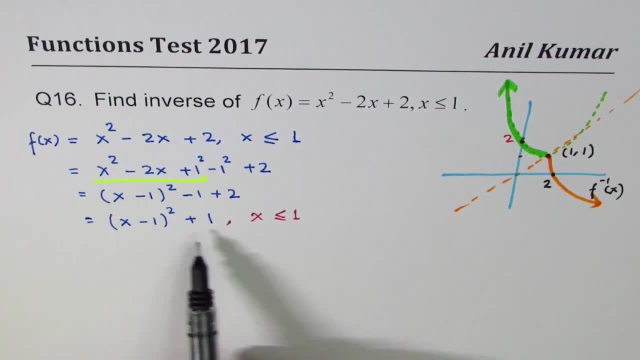 So what we have got here is a parabola, And we are only considering the left arm of the parabola, not the whole thing, since x is less than equal to 1. Perfect, And now let's find inverse right. 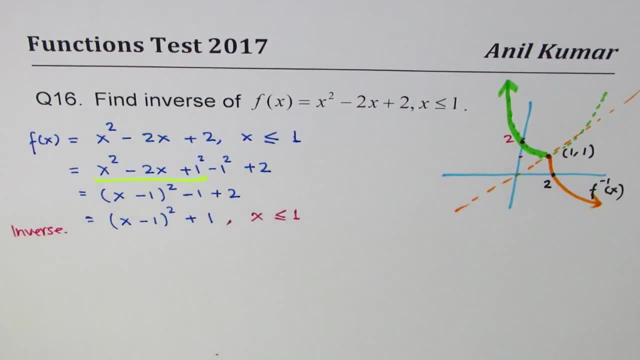 Now let's find inverse. To find inverse, we swap x- inverse, So we can write this as: x equals to y minus 1 whole square plus 1.. Bringing 1 this side, x minus 1 equals to y minus 1 whole square. 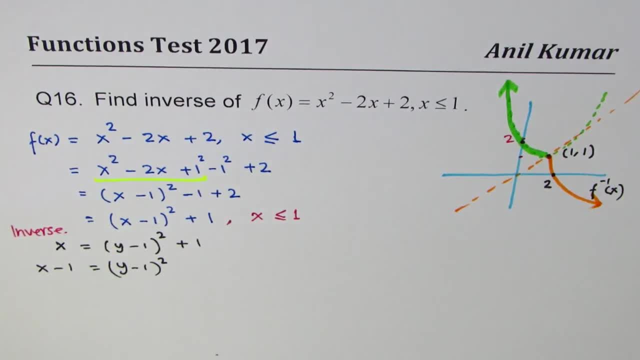 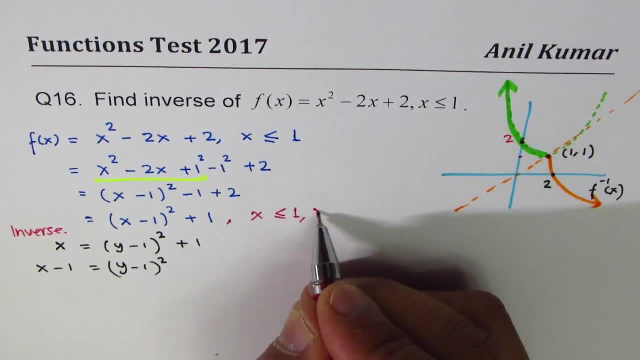 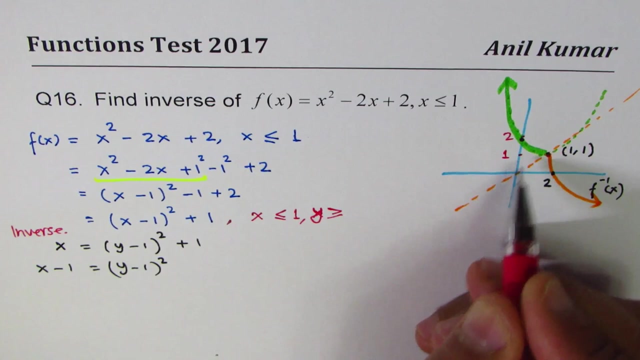 Now remember one thing here. Let me add that also before I move forward, What we observed here is that x is less than 1.. But what is the value of y? y is greater than equal to 1, correct, This is 1.. 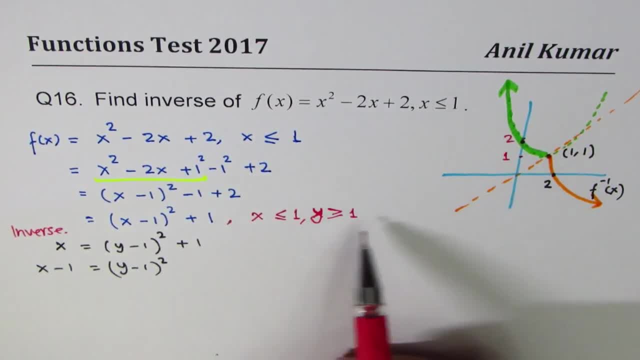 So that's the restriction. So when x is less than equals to 1,, y is greater than equal to 1.. Very clear Vertex is at 1, 1.. Graph opens upwards, Parabola opens upwards. Now, if you find the inverse, then in inverse, what do you expect? 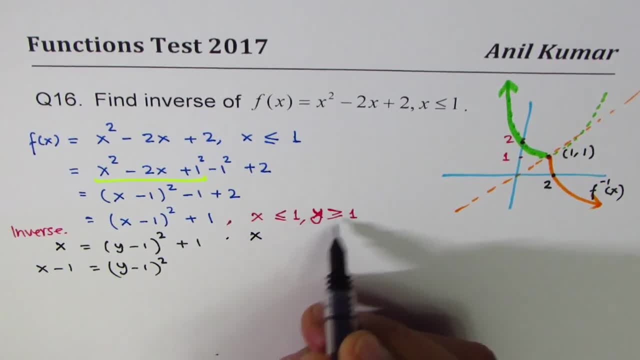 These will change. So for inverse, x should be greater than that. becomes the x value greater than equal to 1. And y will become this, this swap. So for inverse, we swap right x and y. 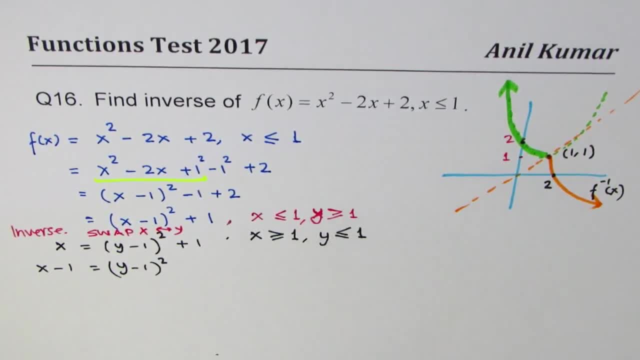 Is it okay? So the domain and range also swap. This is very important to understand, So let's move forward, right? Okay, So we swap x and y, And therefore earlier it was y equals to all this. 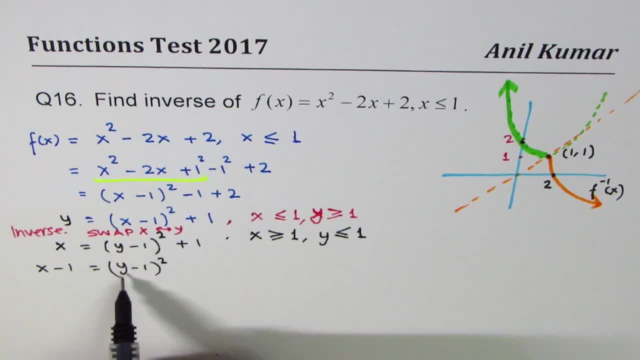 Instead of y we are writing x. So we swap x and y. So we swap y. So we swap x and y. So we swap x and y instead of X. we are writing Y, and now we'll solve for Y. correct, now this is. 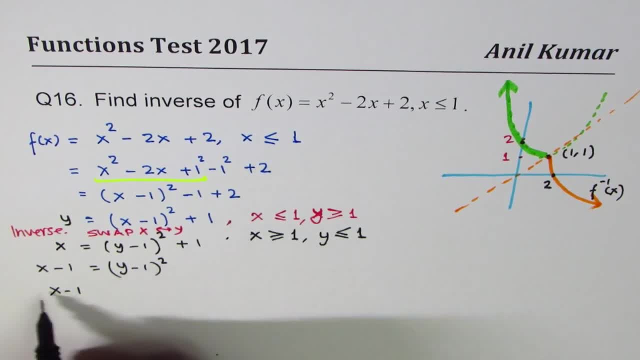 square root: X minus 1. we do square root both sides equals to Y minus 1. square root of squares: Y minus 1. now, since X is less than 1, and whenever we do square, we actually write both positive and negative. right, we actually write positive and negative. however, since we are considering the domain of X less. 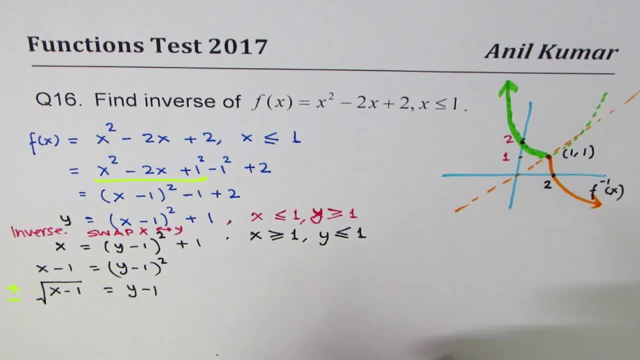 than 1. we are looking only for the negative half, not the positive half, so we'll write negative here, and that is very, very critical to understand. do you get the idea? okay, and now we can solve for Y. bringing one on this side, we have minus square root of X minus 1 plus 1 is 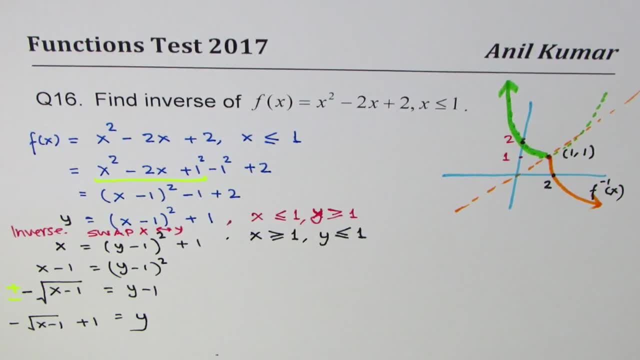 to y. look here. so so let me write down the inverse which we have got from all this so we can write: f inverse of x is equal to minus square root of x minus 1 plus 1.. now look at your inverse function. does it match with the equation? 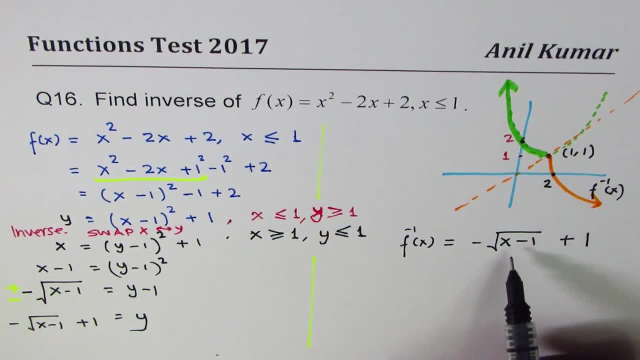 it does, right. so if i write x as equals to 1, this part is 0 and we are at 1. if i write x equals to 2, right. if i write 2, then we get 2 minus 1 as 1. this is minus 1 minus 1 plus 1 is 0, right. 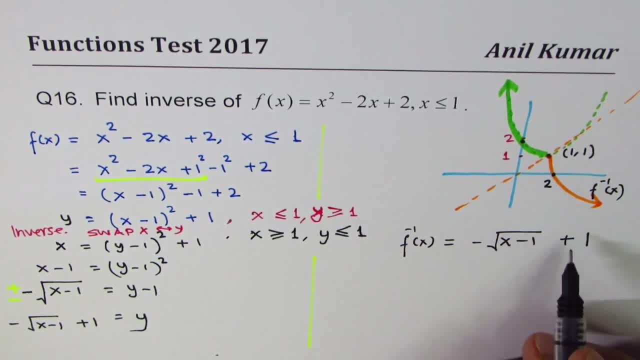 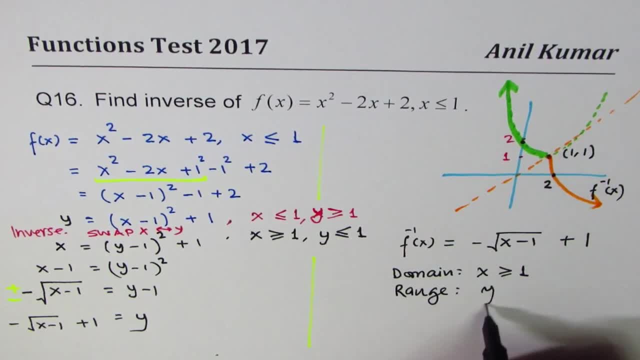 range is concerned, you can see y is less than equal to one, as expected. do you see that? so it's very important in quadratic equations, whenever you are given restriction, that is reflected at this stage. so when you do square root, which sign to take right? so important? so let me write a note.